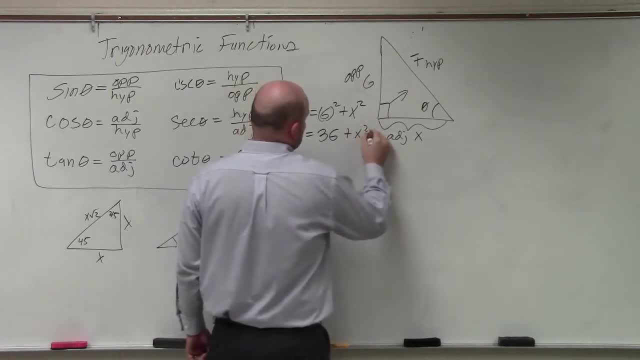 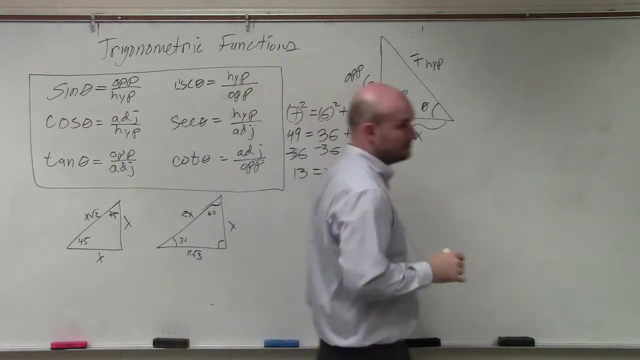 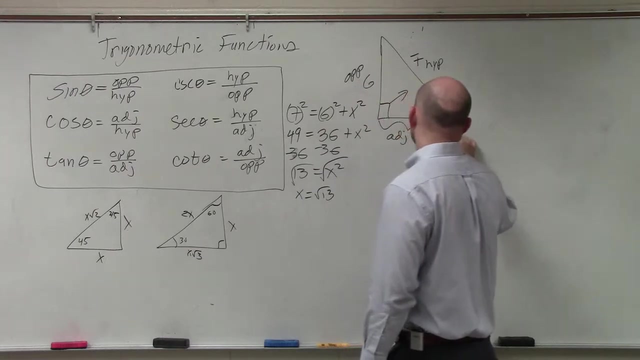 14.. 49 equals 36 plus x squared minus 36. minus 36, 13 equals x squared Right Square root square root. x equals square root of 13.. So x equals the square root of 13.. Everybody. 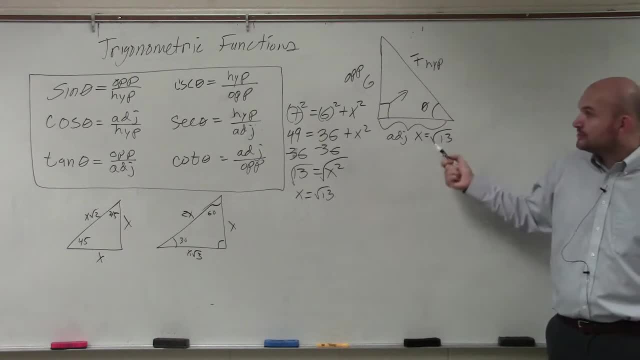 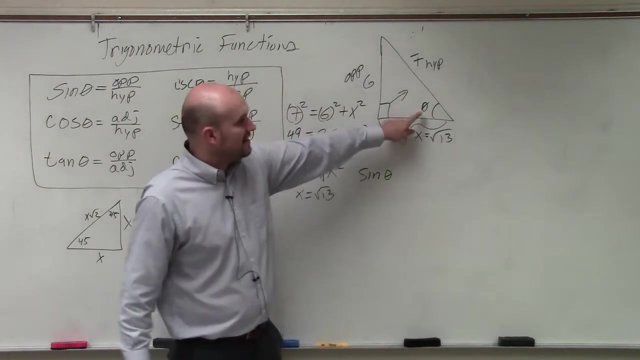 follow me here. So now all we're going to do is we've labeled adjacent, opposite hypotenuse. Now all we do is just do the sine cosine tangent. It's really, you know, not that hard. So now we just do sine of theta, Sine of theta opposite over. 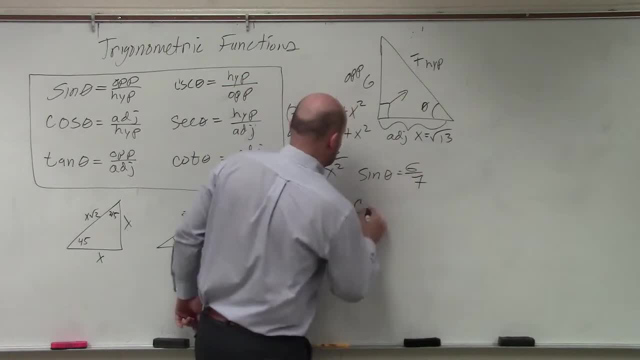 hypotenuse Cosine of theta adjacent over hypotenuse Tangent of theta, opposite over adjacent. So that's 6 over the square root of 13.. However, we don't want to leave the square root of 13 in the denominator, So I'm going to rationalize. 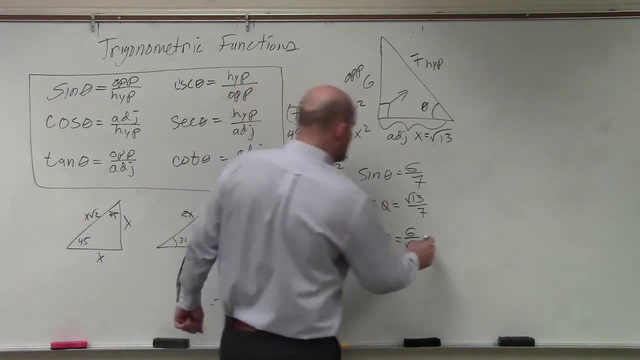 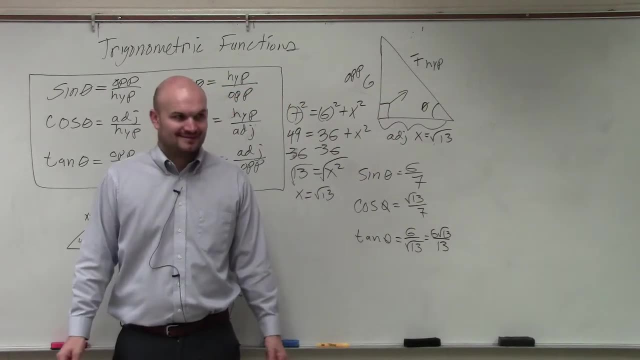 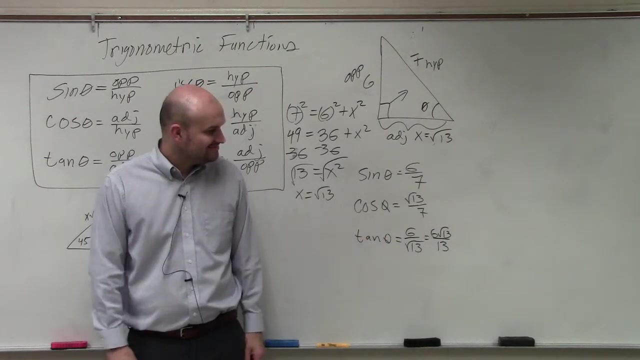 the denominator without showing my work, And let's see if we can get it. Let's see if we can do it in our heads. Does everybody follow me? I just multiplied by the square root of 13 on the top and the bottom Right. Okay, So now that's 3.. We need to find all 6 trigonometric. 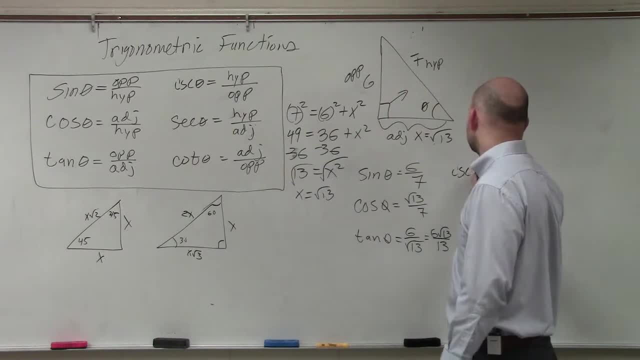 functions. So then we're going to go to cosecant. I always like to do them with the reciprocals, Because now to find the reciprocal of sine is just going to be 7 over 6.. Right, That wasn't that hard. That was very minimal math. 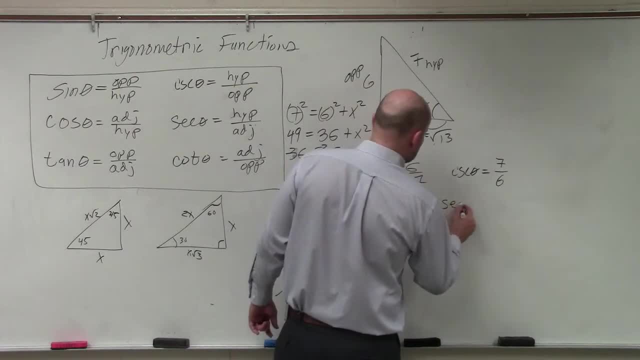 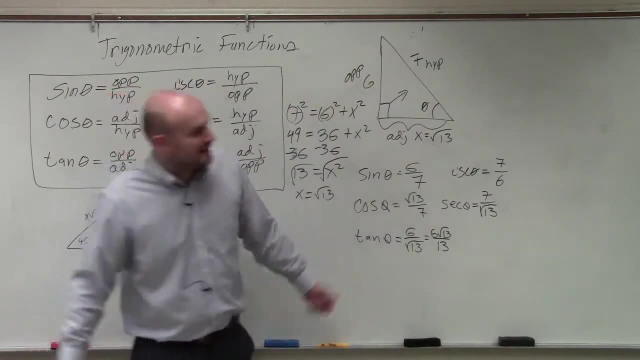 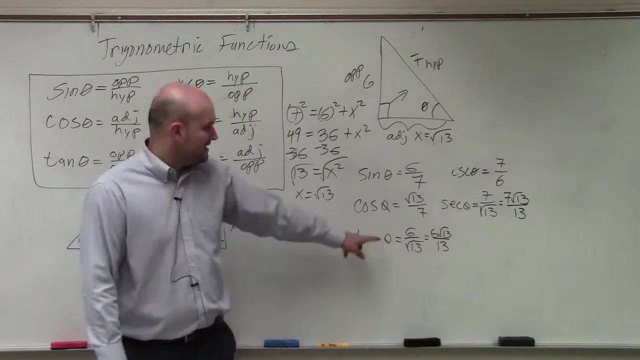 to do This. reciprocal of cosine is secant of theta, So that's 7 over the square root of 13.. Right, But we don't want to write it like that. And then, tangent, I can just write this: Let's reciprocate this. I don't want to reciprocate this one because then I'd have. 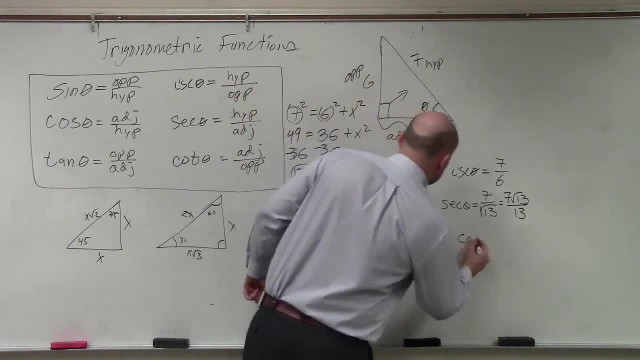 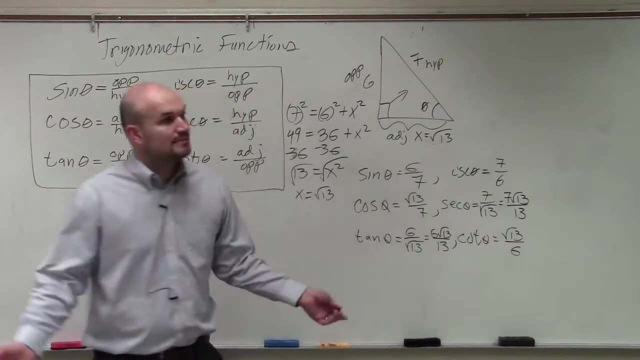 a radical in the denominator, So I'll reciprocate this one for cotangent. That's going to be the square root of 13 over 6. And that's it Done. It's a little bit of kind of tedious work.